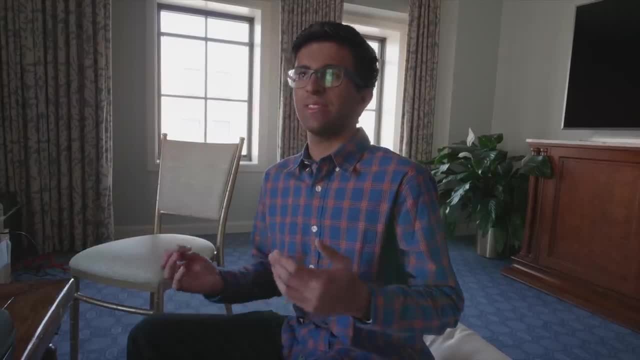 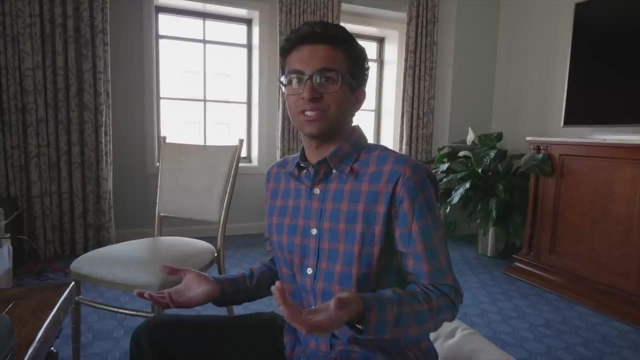 I wanted to make something that you know could fit the greater than half the Earth's population, who, you know, can't just- you know- drive down to an optometrist's office and just get a prescription. So can we see it. 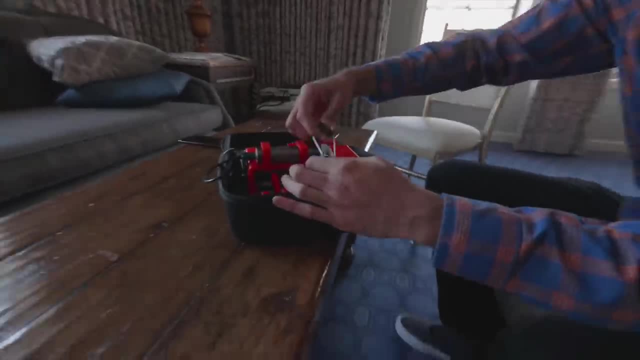 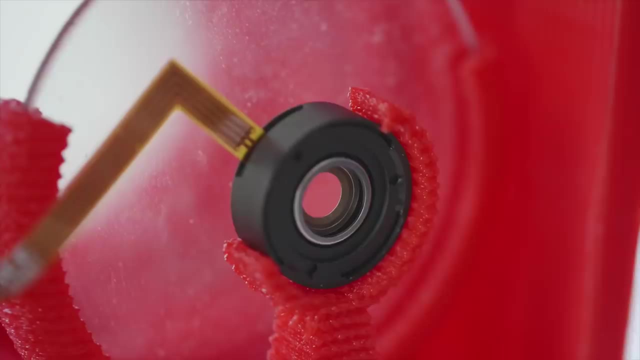 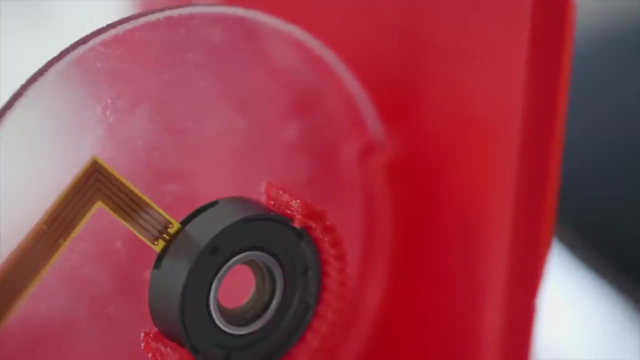 Oh yeah, absolutely. So. this is my child here. This is the portable Phoropter. As you can see, it has the liquid lens that is actually the one responsible for replacing the dozens of precisely machined lenses here. So how does this liquid lens work? 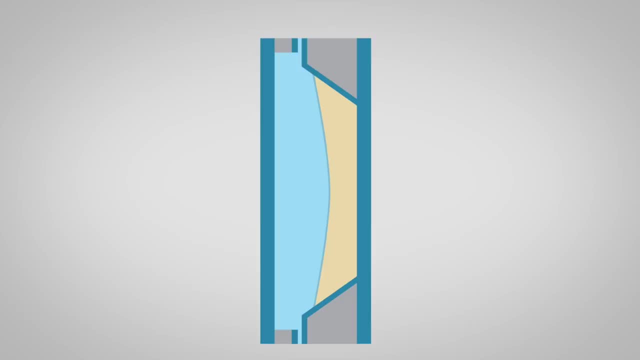 Right. so it has a droplet of a polar substance like water and a droplet of a non-polar substance like a mineral oil. When you apply a voltage across of it, the voltage will be applied to the liquid lens and the liquid lens will be applied to the liquid lens. 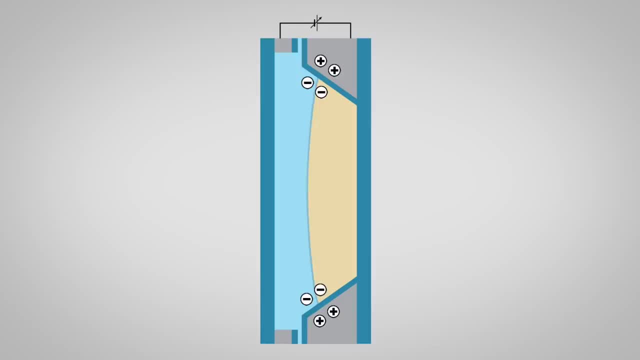 So it has a droplet of a polar substance like water and a droplet of a non-polar substance like a mineral oil. The voltage will cause the polar substance to actually like, change its shape and go, hug or repel the surfaces of the lens. So by changing the shape of the bubble you change the way light. 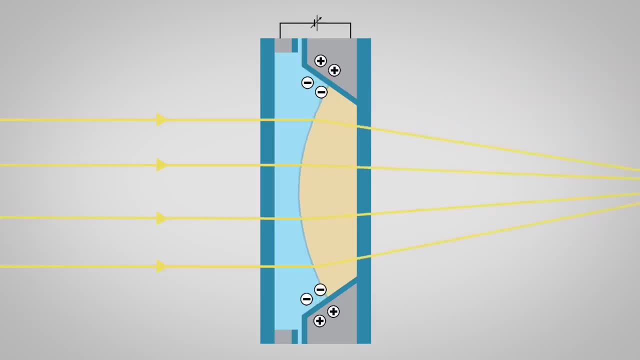 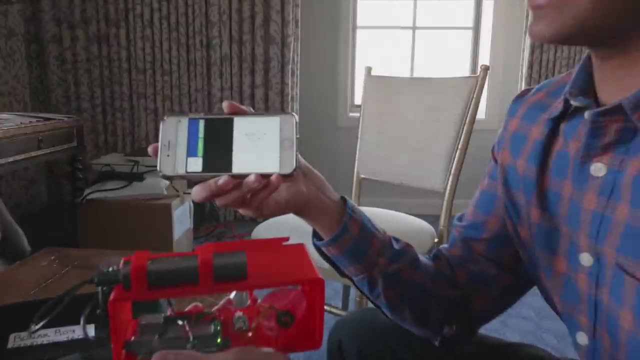 refracts through it as it passes through the two glass windows and therefore you know you're changing the focal length of the lens. You made an app. Yeah, I did So. the screen you're looking at which runs on an app on my smartphone. 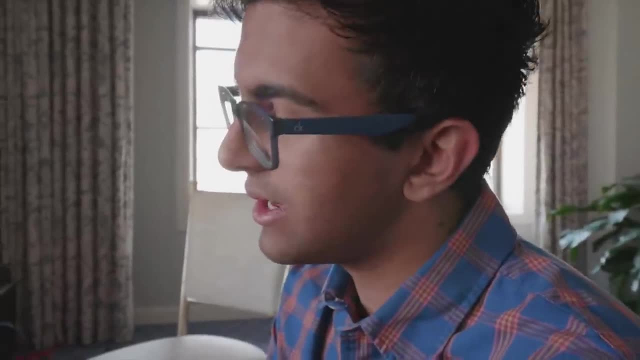 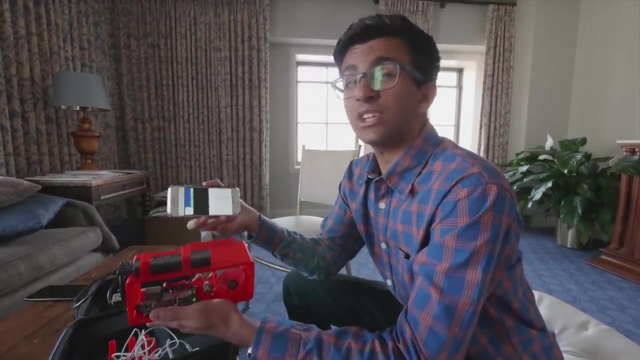 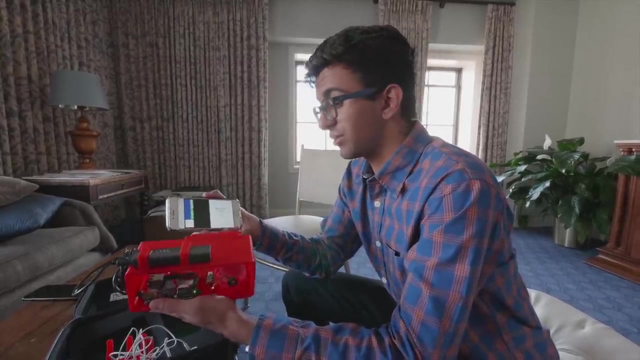 displays a test chart and runs an algorithm to actually do the refraction. I mean, those are pretty small letters Those three static glass lenses are able to make it, so the light coming from the phone are projected to a virtual distance of that 20 feet. So it's basically simulating that test room, but you know, optically instead. 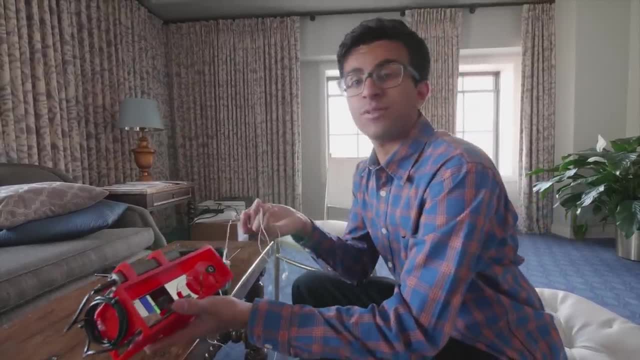 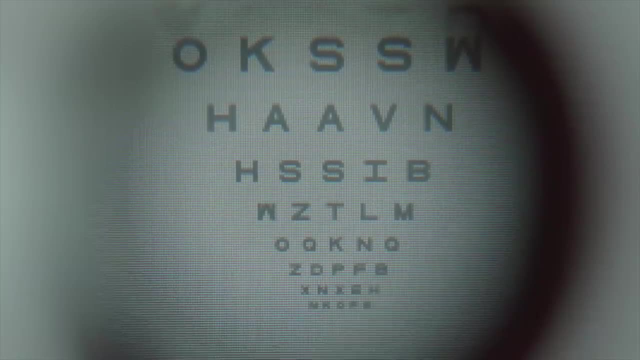 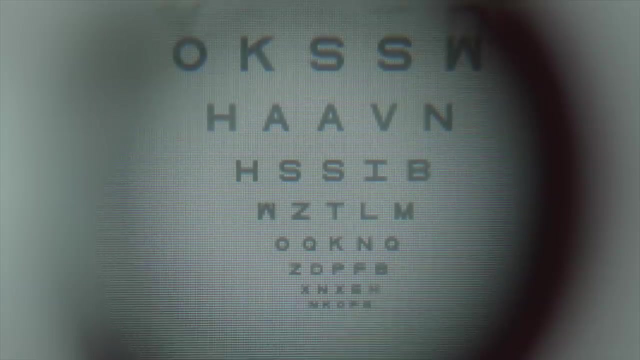 So the way it works is there's an algorithm running on the smartphone app that generates pairs of lens voltages for the patient to compare, And in order to switch between the two lens voltages, the patient can click a button on a pair of headphones. So you can click once to toggle between the two And once you've found which of the 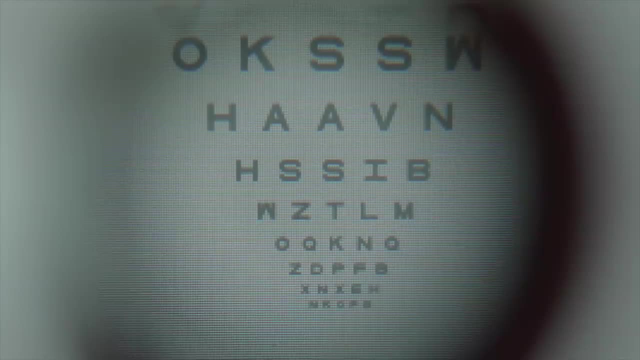 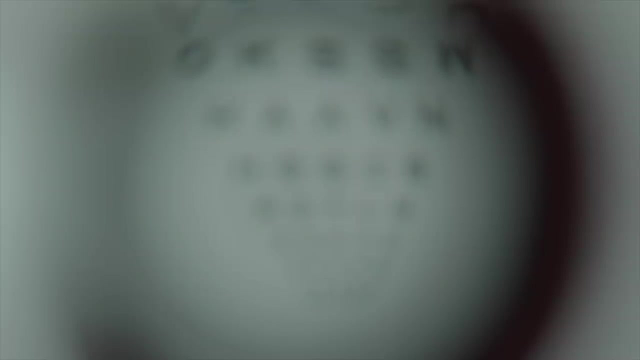 two is the best. Okay, that's better. All right, So you can double click it and it will, you know, indicate to the algorithm that it indeed is the best and generate the next pair. Oh, I think it got worse. 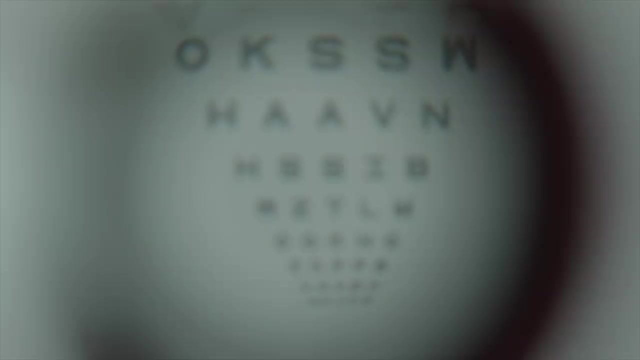 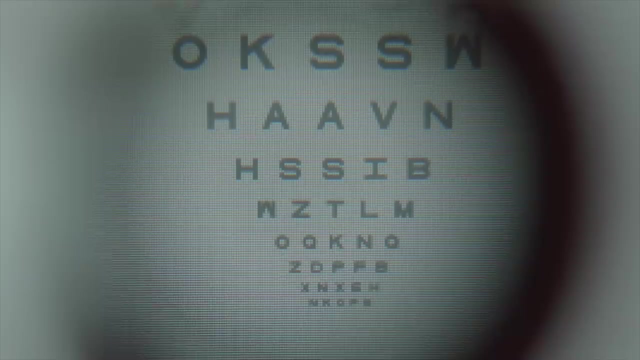 Yeah so, And I'm going to click Uh yeah, Okay, that's better, but it's not the best I've seen. The algorithm will basically cycle through this lens voltage pair generation process. This is like night and day, It's not even a question. 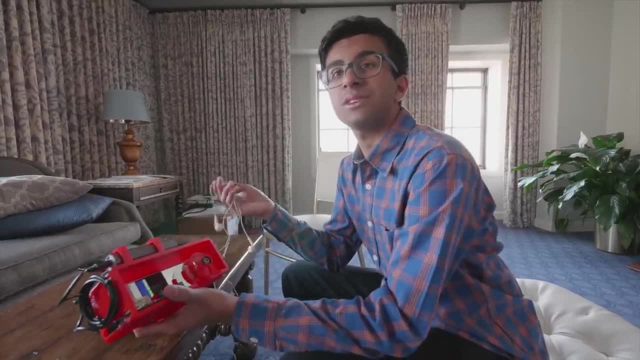 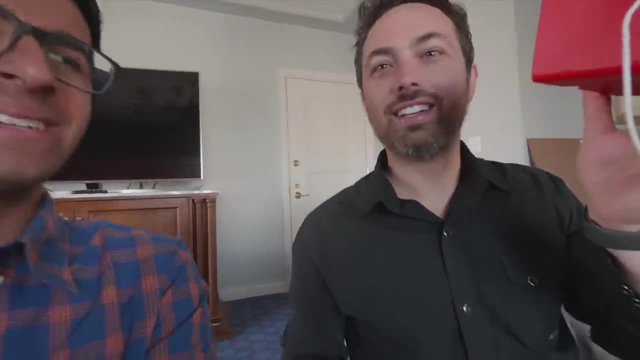 Until it zeroes in on the one voltage that works best for you. Okay, Okay, that, or Aha, yes, Test complete. All right, awesome, Would you like to know? I would love to know what my eyesight's like. 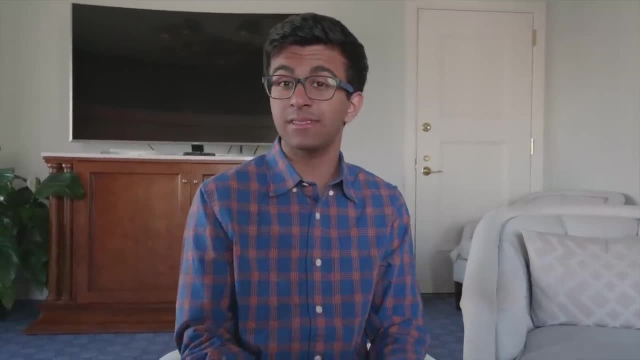 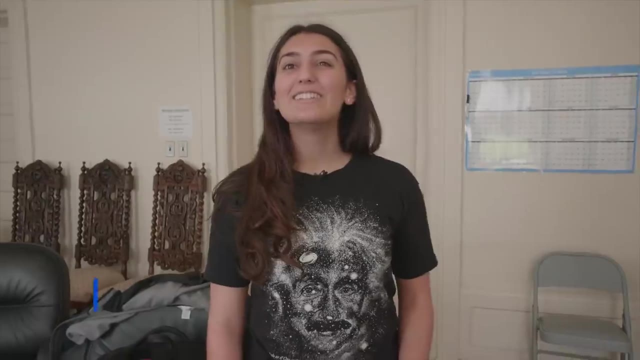 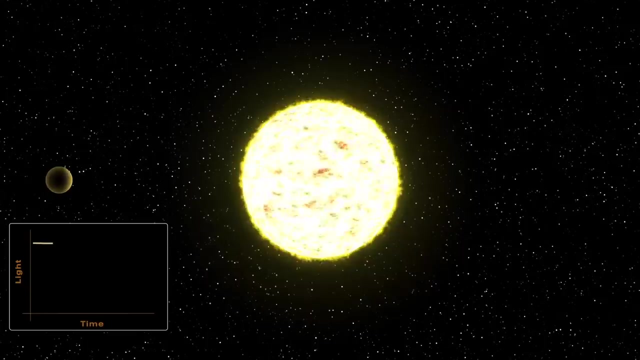 All right, So I calculated negative 1.25 diopters, which is roughly in the range that most people with slight nearsightedness would have. Anna Humphrey wanted to find hidden exoplanets with math. The Kepler Space Telescope has been the most prolific planet finder to date. 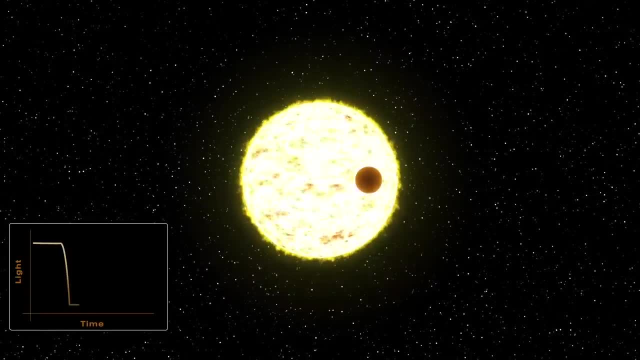 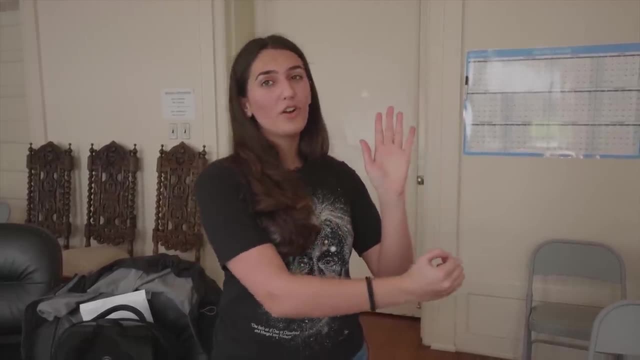 detecting over 2000 exoplanets. The Kepler Space Telescope has been the most prolific planet finder to date, detecting over 2000 exoplanets by measuring a dip in their host star's brightness when they pass in front of it. But what happens if the planet passes just above or just below the star? Also, what if that planet is really small? Those little tiny shadows are really hard to pull out when you've got a lot of noise. A further challenge is that the Kepler mission only ran for four years. That means our absolute limit is. it's really hard to find anything that takes longer than four years? 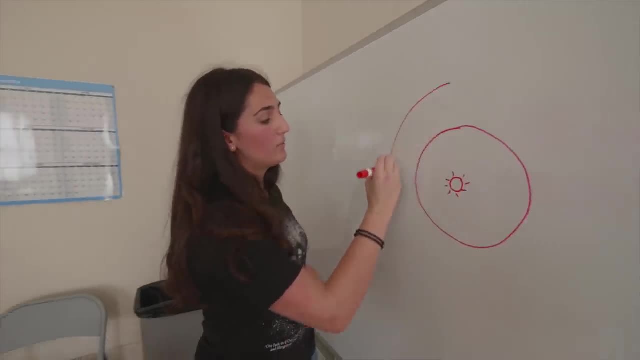 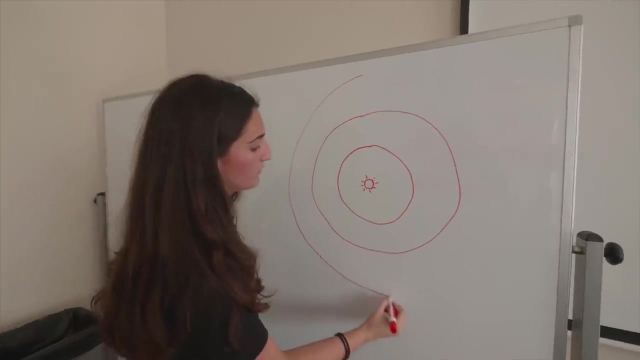 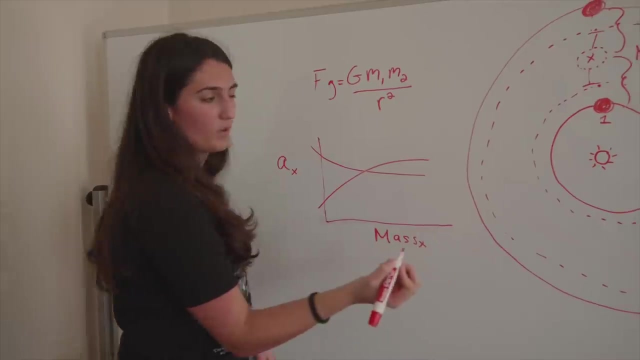 to orbit To identify planets Kepler might have missed. Anna has been working on a new model of measuring multi-planetary systems and calculated whether additional planets could fit in between the ones we observed without disturbing their orbits. I imagine that you already have some sort of planet here, so we're going to call this planet X. 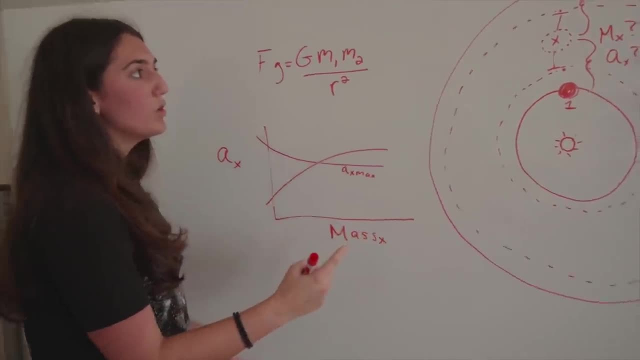 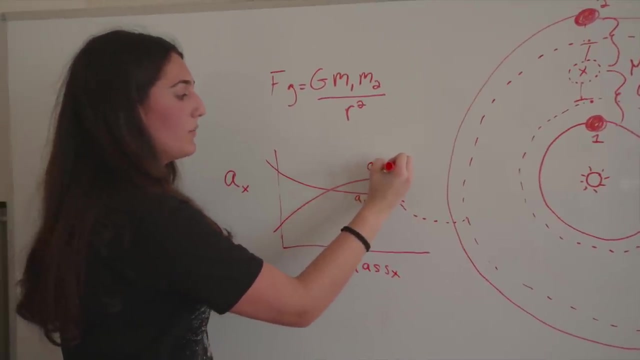 So what are these two lines? This line here is the same as this outer line, It's how close the your imaginary planet can get to your outer planet. And this line here is your AX min. It's how close your imaginary planet can get to your inner planet. 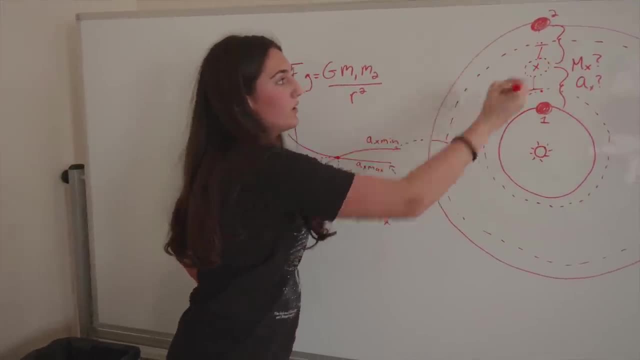 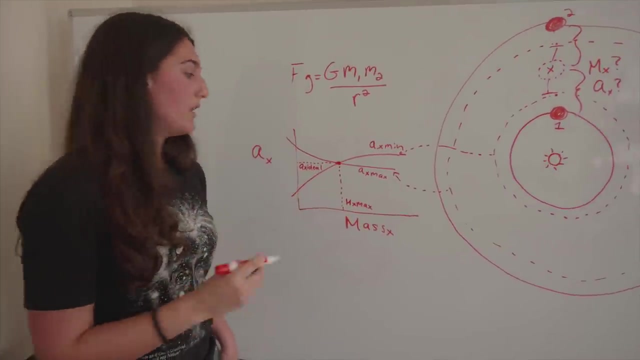 So it's this line. here We have this region of stability, given the extremes of where we can put a planet And we have the maximum mass that you can fit there And anything in this area here sort of shaded around our label. 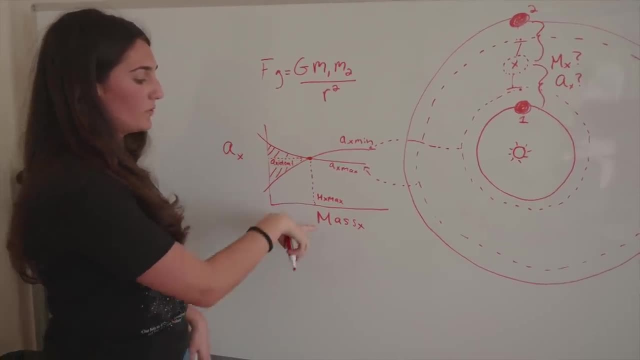 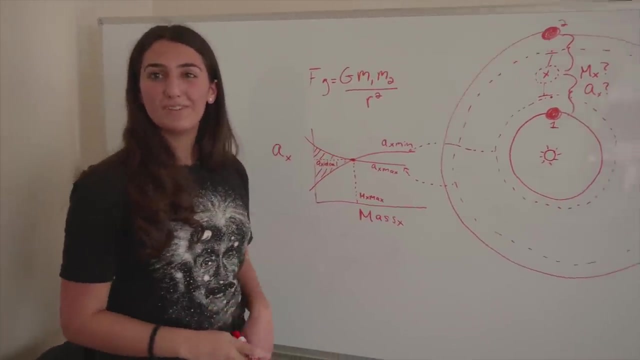 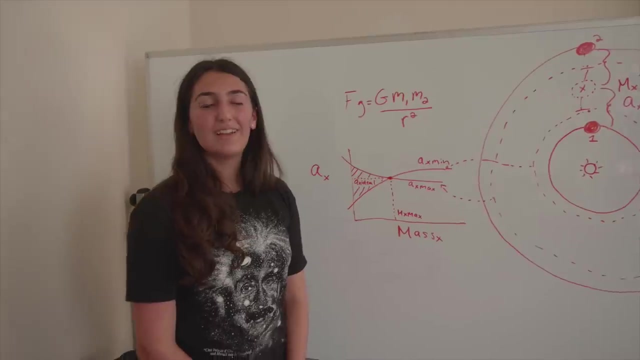 anything between these two graphs is a combination of a planet's mass and a location of the planet that we could fit in between the two we know about and maintain a stable system. Cool Yeah, Now the question everyone will ask you is: like what's to say that this planet really exists, as opposed to you just making up stuff? 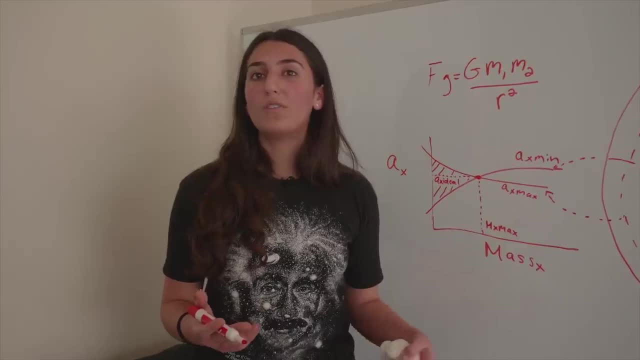 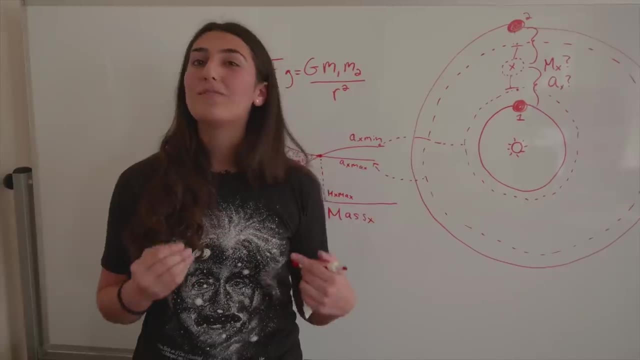 So the assumption that I made going into my research was that systems are going to try to have as many planets packed in as possible. This is called the packed planetary system hypothesis. There are 560 locations where we could fit additional planets, so quite a few. 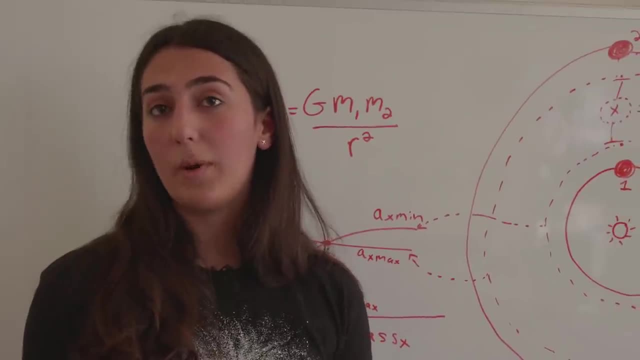 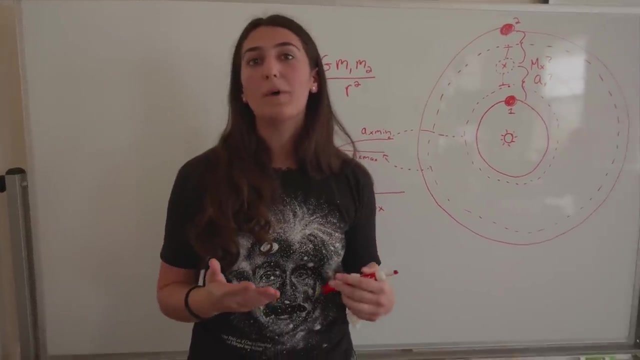 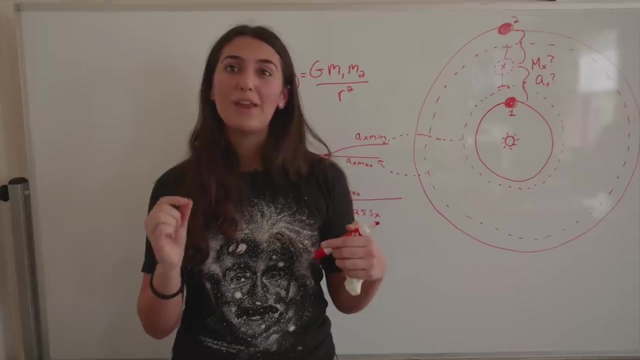 How might we go about actually finding them? One of the ways you could go about doing this is by doing something called folding the data. So let's say we figure out that a planet should have an orbital period of about one month, We have a year's worth of data, and we fold that data in 12 and get it to line up just right. 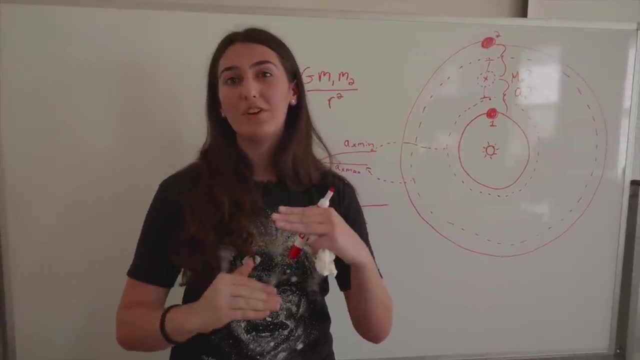 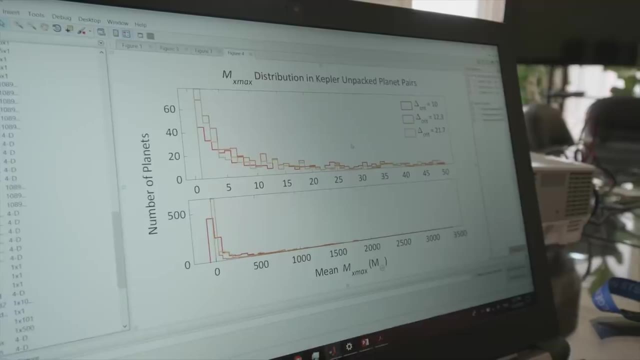 We can get it, so those transit signals actually layer on top of each other And then we get a larger signal that we can find, as opposed to the really small signals that sort of get lost in the noise. Do you want to introduce yourself? 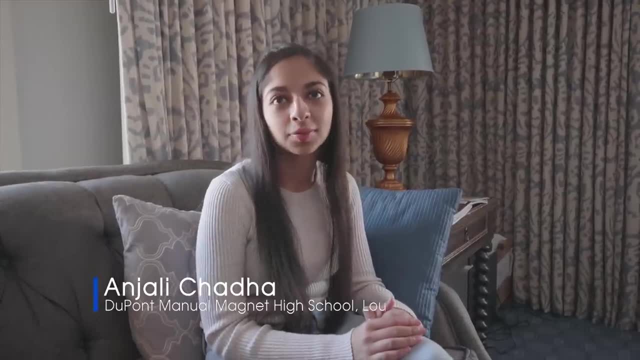 Sure, What's your name? What do you do? Yeah, My name is Anjali Chaudhary. Hi Hi, Hi. I am a senior at DuPont Manual High School in Louisville, Kentucky. What is this? Some of that. 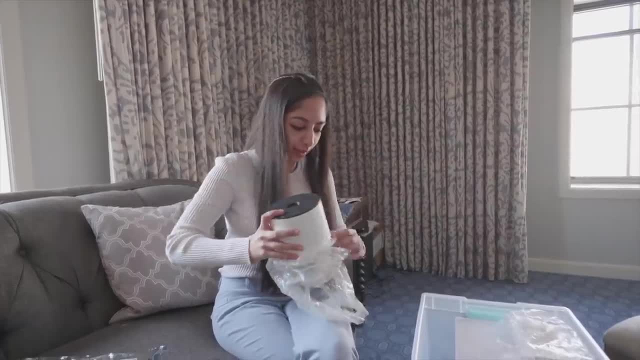 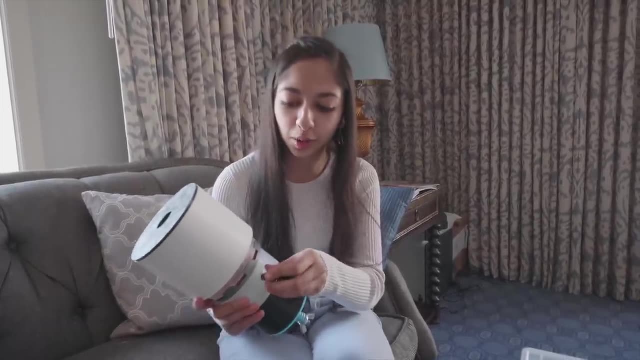 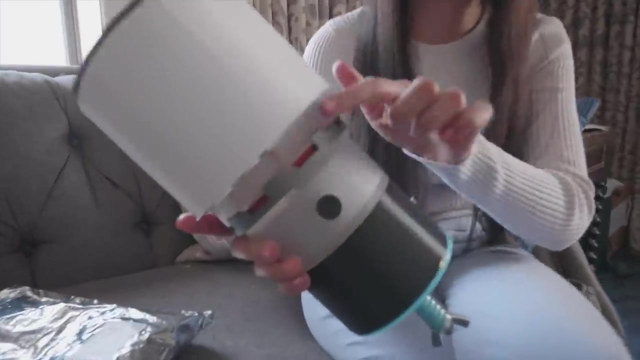 Anjali was concerned with dangerous contaminants in drinking water. This is a prototype of my arsenic sensor, So you want to load a water sample right here in this compartment. The whole process starts with an automated chemical reaction. So there are a bunch of chemical reagents that sit in this compartment above the water sample. 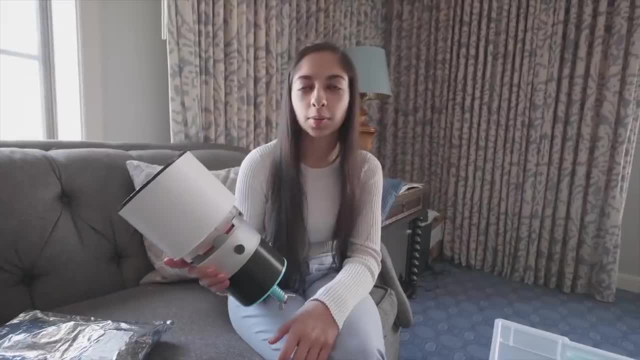 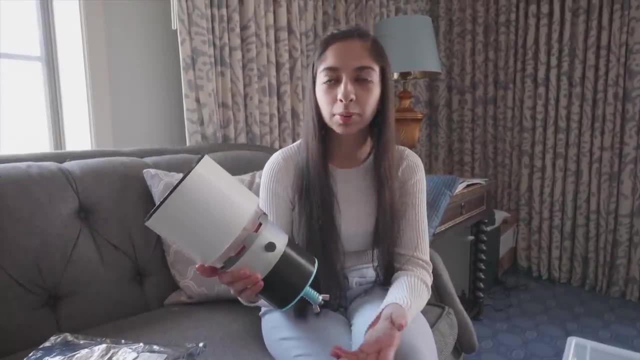 So the first reagent is tartaric acid, Next is a combination of salts- It's called monotacium sulfate- And then the third is zinc. Arsenic is an element that's never found freely, but it's always bound to other elements. 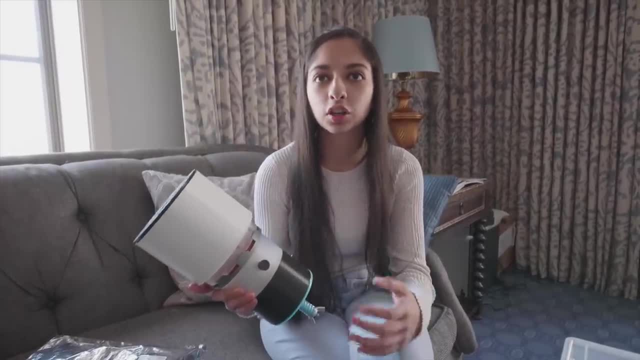 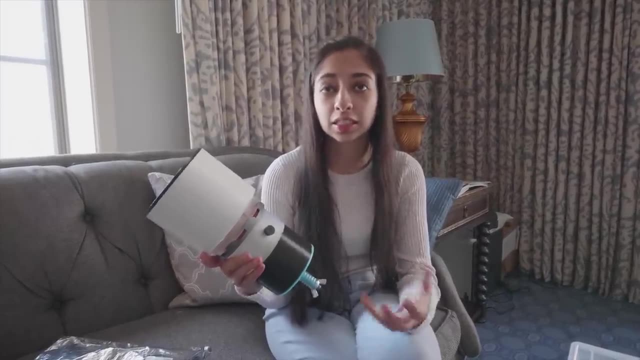 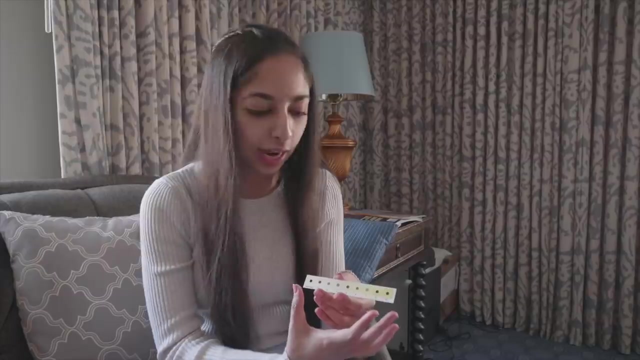 So basically, that chemical reaction will help to free up all of the arsenic And then the arsenic content changes into a gaseous form of arsenic gas And that's the best detectable form of arsenic, basically. So what happens after that gas is formed is that there is a test strip and it's covered in mercury. 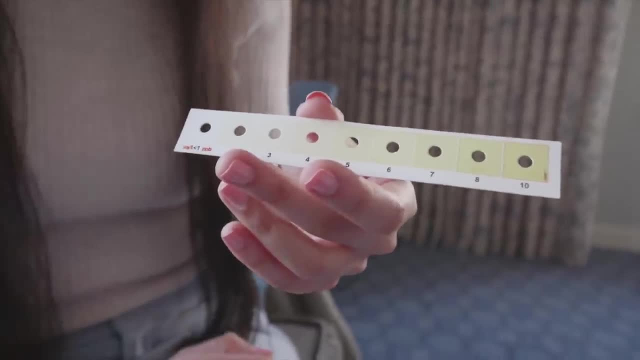 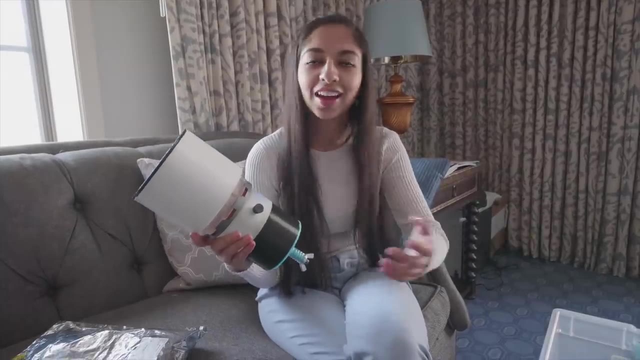 bromide which oxidizes in response to the arsenic and then changes color. So it's actually on a gradient scale: If there's very little arsenic content, then it changes to a light color, And if there's a lot, it changes to a dark color and everything in between, right? 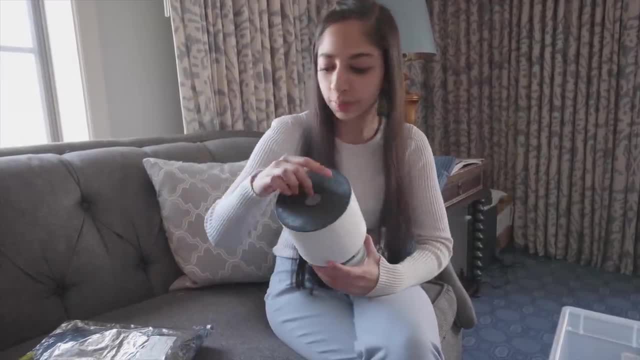 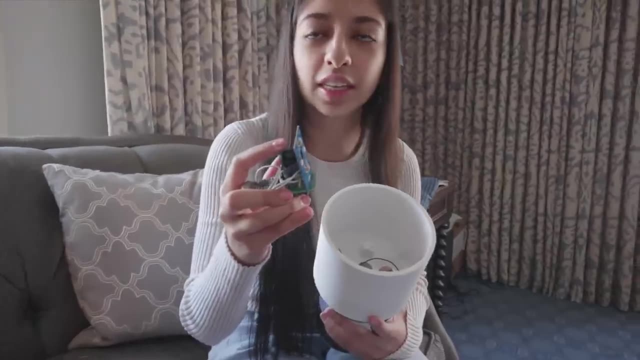 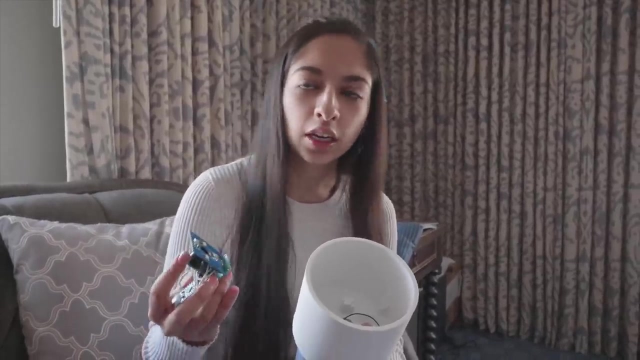 So what I then did was write an image processing algorithm using some embedded electronic devices, specifically this device called an Arducam. It's just an embedded camera, And essentially the camera takes a picture of that test strip After it's changed color. it then pulls out all of the color values of the test strip. 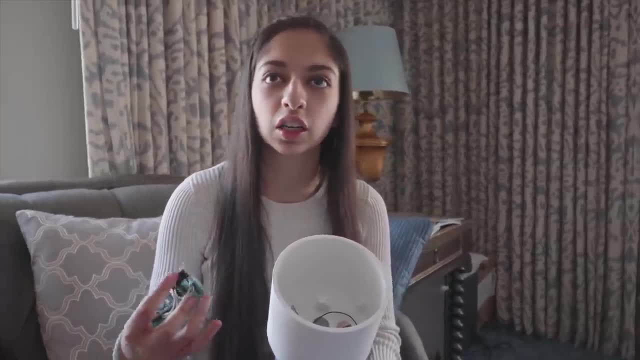 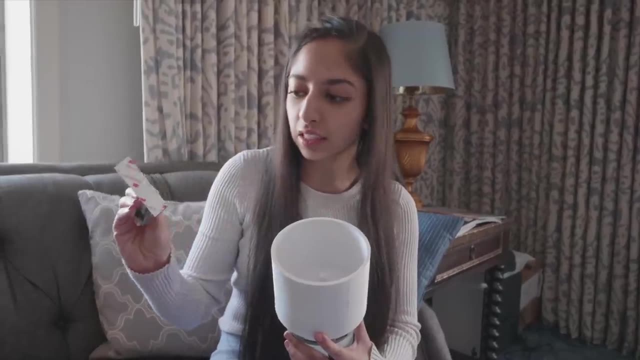 and converts them into concentration data. So I wrote some mathematical models that kind of make that conversion. And then the last kind of piece of the puzzle is that there is this device: It's a microcontroller called a particle electron and it's connected to this cellular antenna. 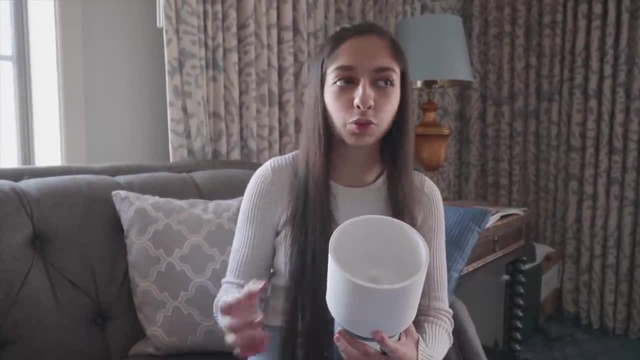 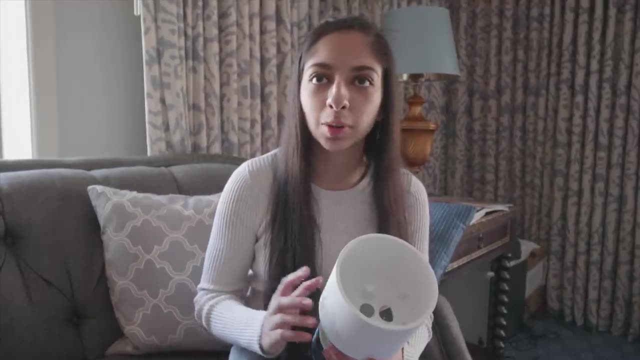 so that the data is instantaneously transmitted to the cloud, And the real advantage of that is that several people would be able to access the data collected from one sensor, Whether it's people in the same community who want to kind of have that information and knowledge about their water sources, or whether it's people in research organizations. 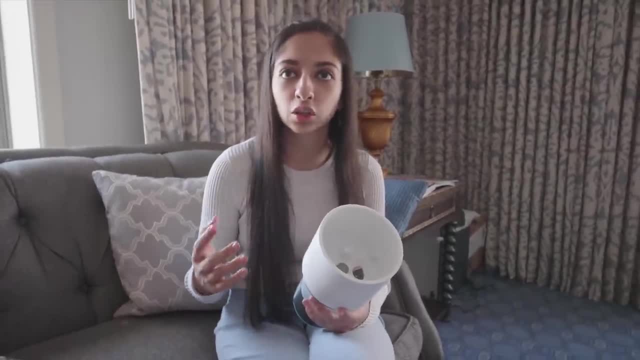 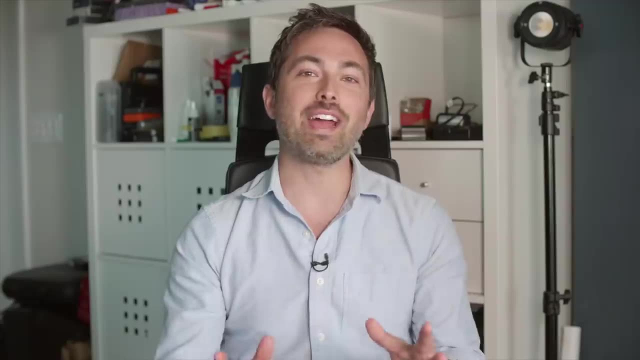 who are trying to really learn more, learn what to test, learn what to improve and what sites to really work on. So those are kind of the reasons why I chose to do that. So now the moment of truth. Which one of these high school students will win $250,000?? 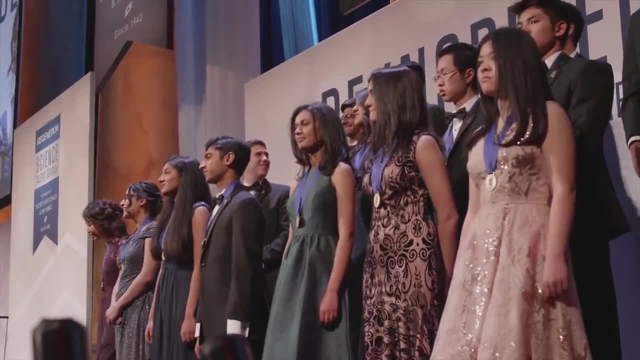 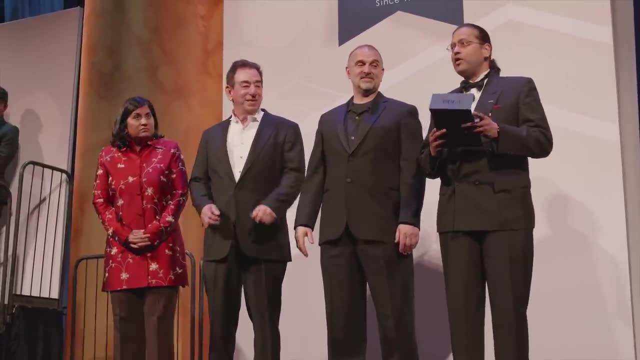 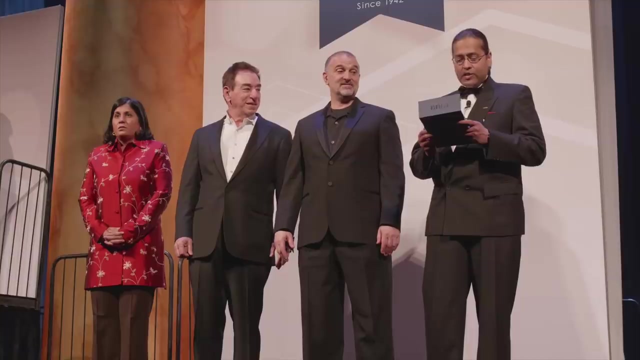 Now I should point out that all 40 finalists each receive at least $25,000, with the top 10 receiving more than that. The first place winner and recipient of a $250,000 award from TC Williams High School in Alexandria, Virginia, Anna Humphrey. 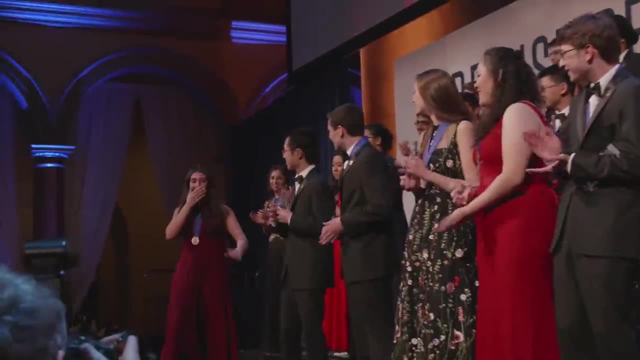 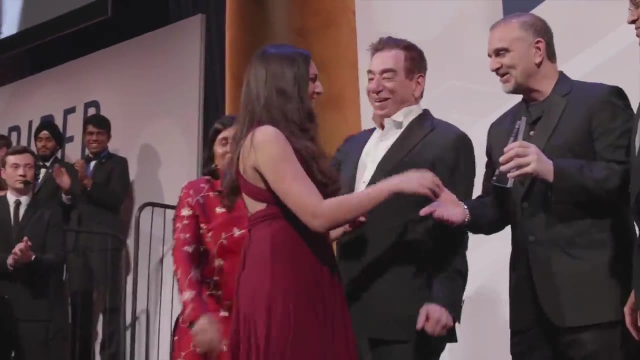 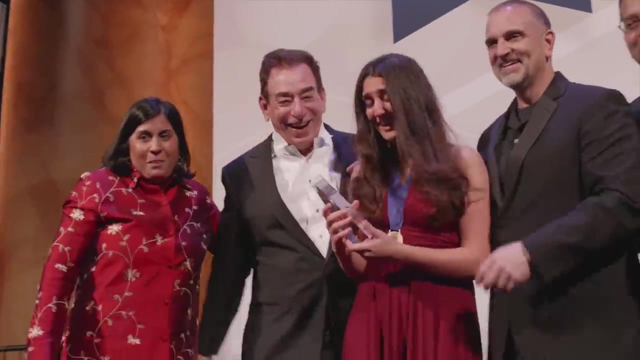 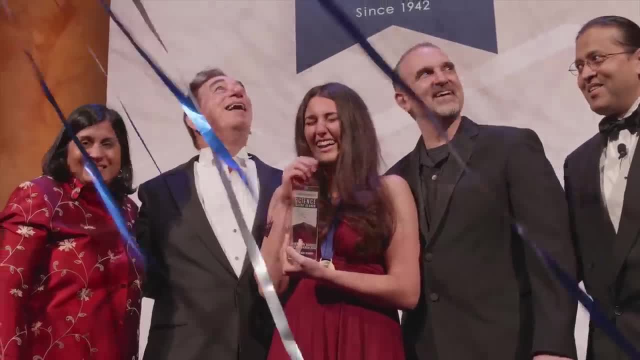 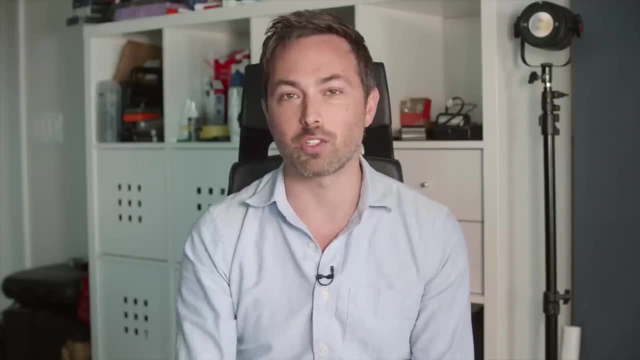 video. It could be their turn next up on that stage. And if you are an American high school student, think about these numbers. Around 3.6 million students graduate high school in the US each year, but only 2,000 or so apply to the Regeneron Science Talent Search. 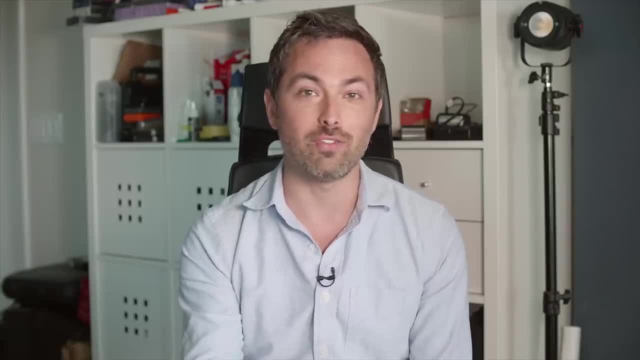 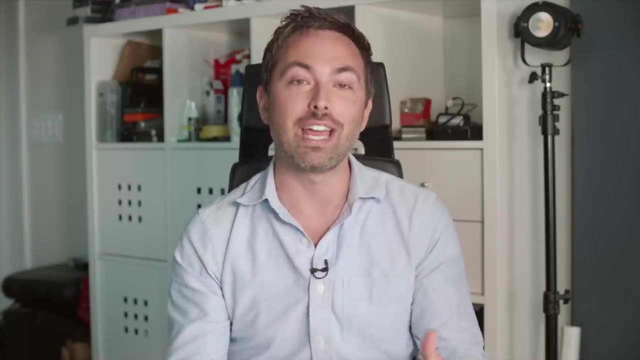 That means if you enter your science research project you have a 1 in 50 shot of winning at least $25,000.. I mean, when else in high school do you get the opportunity to get such a financial boost and receive recognition for your ability in science and math?